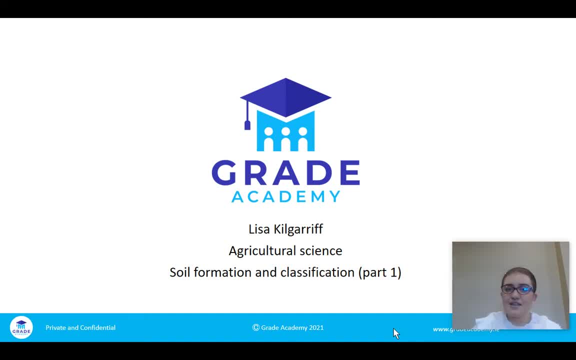 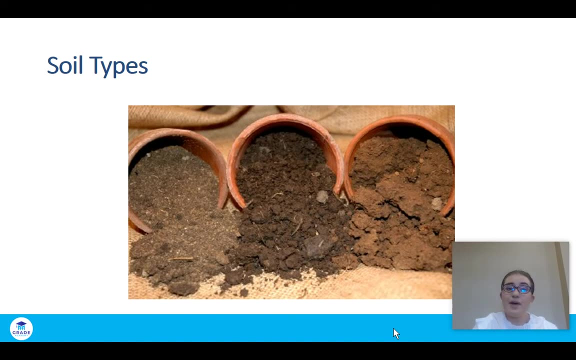 Hi, my name is Lisa Kilgariff and welcome to this Great Academy lecture. In today's lecture, what we're going to look at is soil formation and classification, part one of that. So, in relation to soil, there are many different types of soil. Some soils are more fertile, some soils are better. 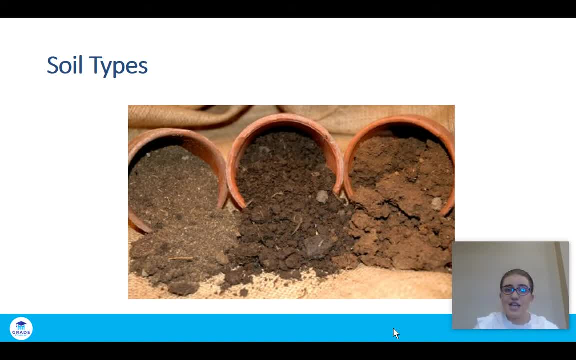 at heating up, and some soils are more suited to tillage grazing, other ones are suited to forestry. So what we're going to explore in, really, this first section of the course is soils, The different characteristics of them. what makes a good soil, what makes a soil? maybe that would 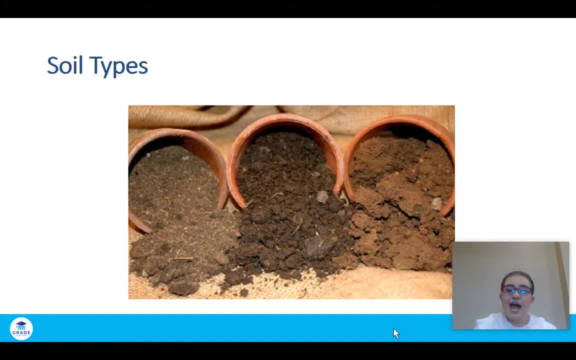 need a little bit more encouragement due to fertilizers and all of that kind of stuff. And if you look at the picture here on the first slide, you can see very distinctively there is three different types of soils here, So the colour is different. we can also see that in some of the 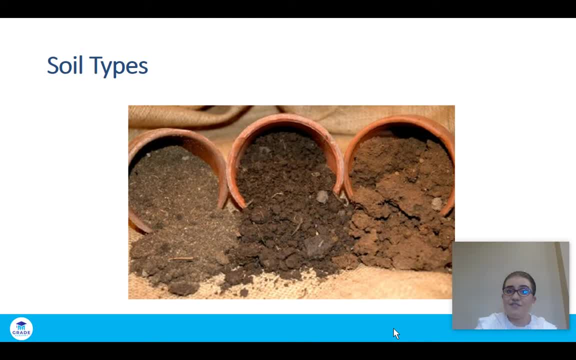 soil samples here. they're grained up quite finely and we'll be looking at that. We'll be looking at two main types of soil. We'll be looking at clay soils and we'll be looking at clay soils and we'll be looking at sandy soils and the different size of the particles in those. You can also see there's. 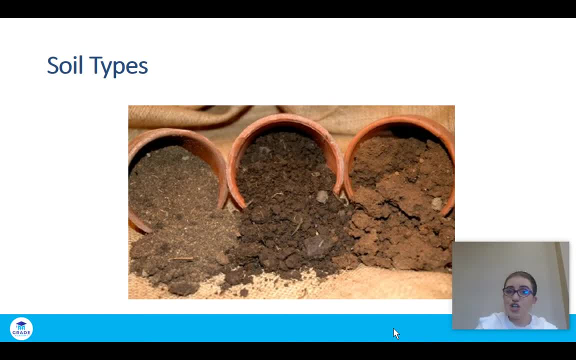 some clumps in some of the soils, and again, to a certain degree. yes, you do need a soil structure and you do need a certain amount of clumps, but too much clumps is going to lead to waterlogging, it's not going to allow air to move freely through the soil, and so therefore, that's going to prevent. 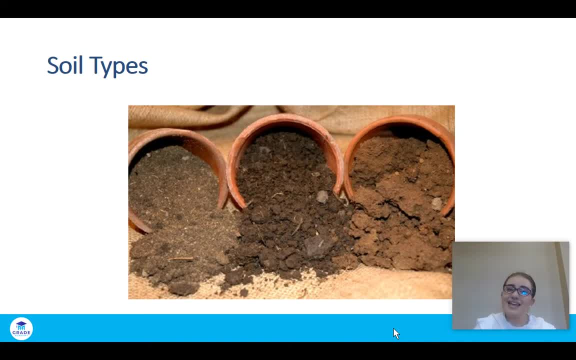 growth from occurring. So that's really what we're going to be looking at. but before we kind of get into soils, what we need to do is we need to look at the parent rock underneath the soils, and that's what the next lecture is about. So we have three different types of rock. We have igneous. 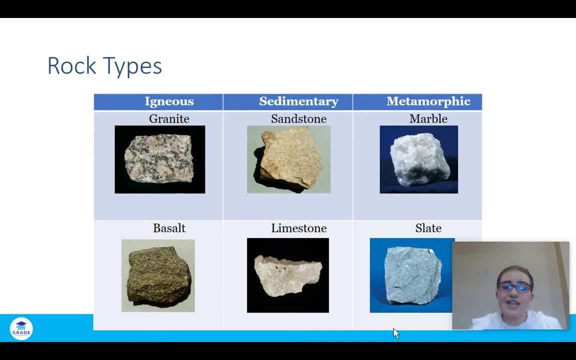 sedimentary and metamorphic rock, and what's really important is that you know briefly how each of them has been formed and an example within each. So within igneous, we have granite and basalt, Within sedimentary, we have sandstone and limestone, and within 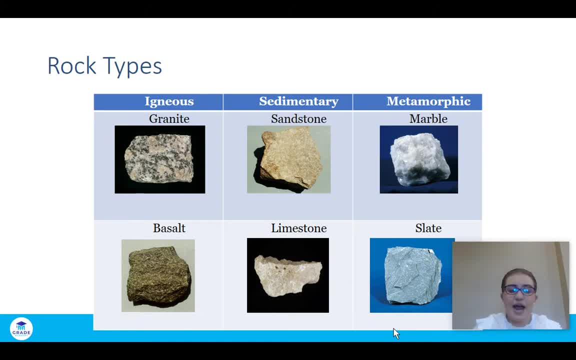 metamorphic. we have marble and we have slate. So depending on different areas, you know where ever you are in the country- the parent rock will be different. So in certain areas igneous rock will be quite prominent, in other areas sedimentary rocks, and so on and so forth. 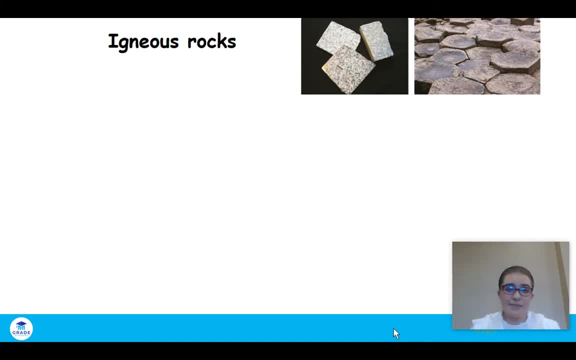 So, looking at igneous rock first of all- and igneous rock, the main two examples that we look at there are basalt and granite. Okay, so how did igneous rock formed? And the way I always think about it is three different types of rock- is sim, So think of the sim card for your phone. 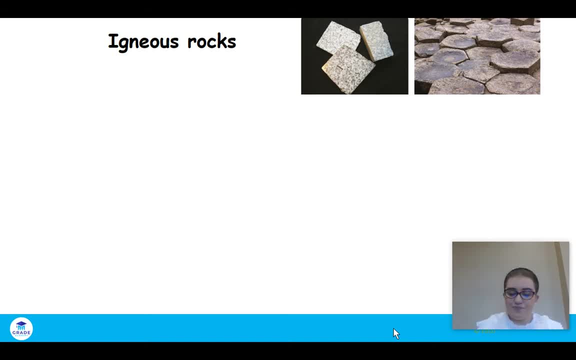 I for igneous and M for metamorphic. So these are the first rocks ever formed on earth. So they, you know they have been around for quite a while and when we look at metamorphic rocks, we look at that- the fact that igneous rocks play a part in forming the metamorphic rocks. 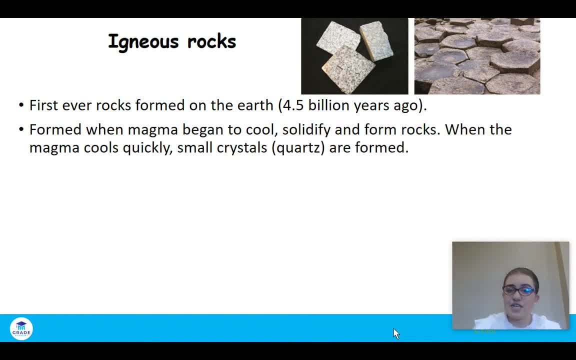 So they formed when magma cooled and it's solidified, and how it's solidified will form the different types of igneous rock. Okay, when the magma cools quickly, small crystals will form. So depending on how the magma cools, different size crystals will form in the igneous rock. 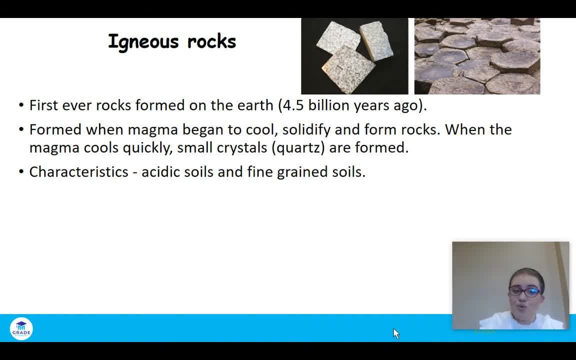 The characteristics of it. generally, where you have igneous rock, you will have acidic soils. Okay, and acidic soils generally means that the pH of the soil is less than seven. If we look at an alkaline soil, the pH is greater than seven, And we'll also see 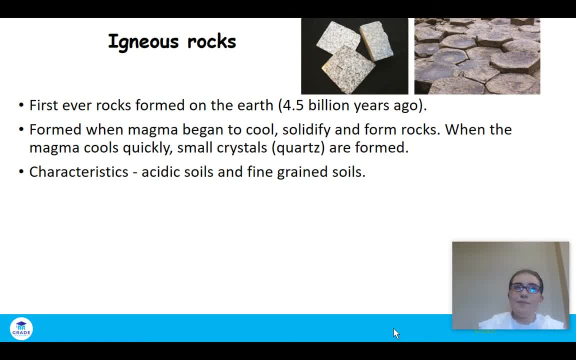 that with finely grained soil. So finely grained soils, to a degree, are quite good in relation to nitrogen and everything like that. but the problem with finely grained soils is that they will and they can kind of clump together and they can lead to water locking. So it just depends. 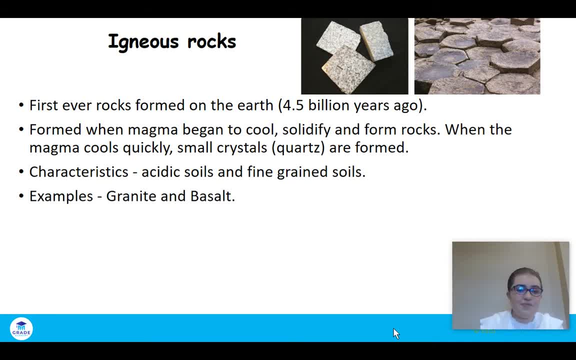 on how the land is maintained, to kind of prevent that. So the examples, as I've said already, are granite and basalt. So how did granite form? So granite cooled very slowly and gave large crystals, all right, and it's also acidic. Basalt cooled faster and 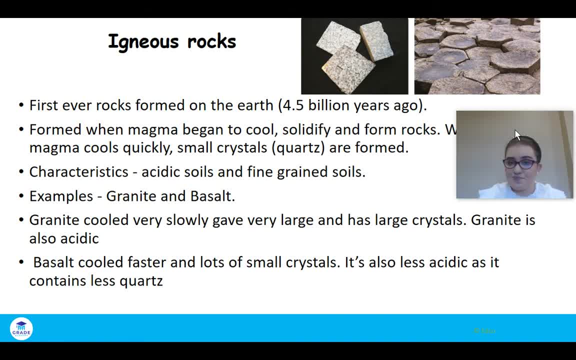 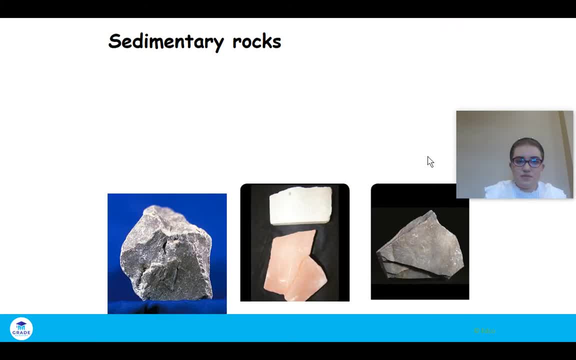 basalt cooled faster and there was lots of smaller crystals formed with basalt, So that's igneous rock. The next type of rock that we're going to have a look at is sedimentary rocks, So sedimentary rocks formed from sediments or from particles deposited in seabeds and lakes. 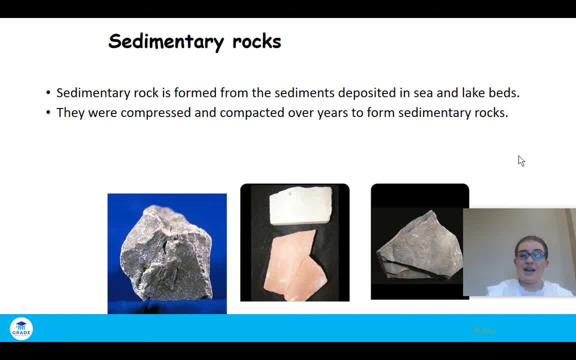 They were compressed and compacted over many years. So compressed and compacted means that they're this great presence of sediment. They were compressed and compacted over many years. So compressed and compacted means that they're this great presence of sediment. So compressed and compacted means that they're this great presence of sediment. 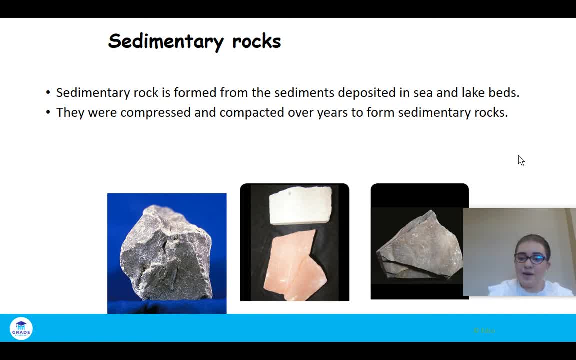 And you're going to have, you know, fossils. you're going to have different sediments and over time there's great pressure and from different layers building up and that's how sedimentary rocks formed. So when you look at sedimentary rocks such as limestone, a lot of the time you actually find um kind of fossil remains in them. 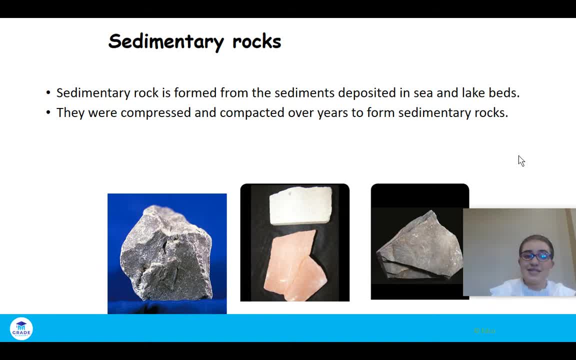 simply because that's how they've been formed and that's where the name comes from. So sediment, sedimentary rocks. Examples include sandstone, limestone shale, So I suppose one of the main areas where we would see limestone is in the Burren and County Clare, so that's a huge area. 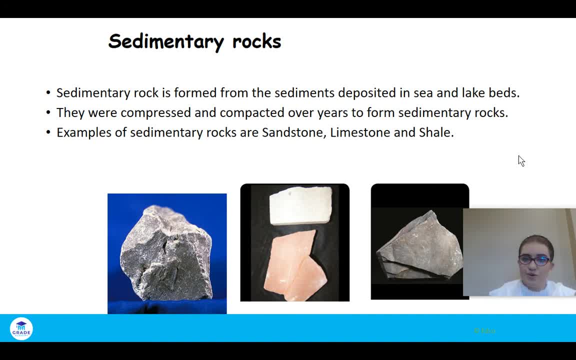 of kind of exposed limestone and not really useful for agriculture but there is. it's very important for biodiversity because you do have quite a lot of unique animals and plants living there and but in terms of like grazing, tillage, things like that, it wouldn't. it wouldn't be that useful. 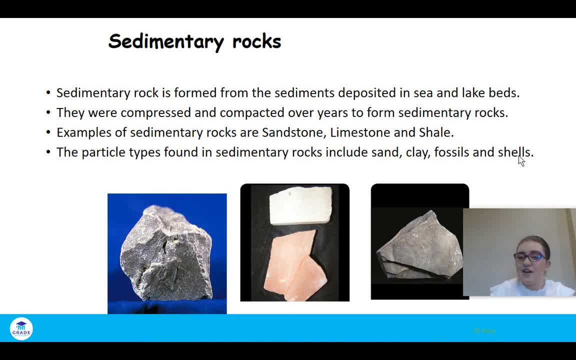 So the particle types found in sedimentary rock include sand, clay, fossils and shells. so really, what's important for sedimentary rock is that it is the sediments, or small little particles compressed over many, many years, and you can see some examples of them there: Metamorphic rocks. 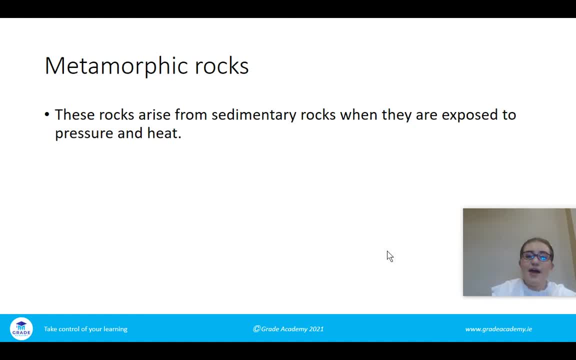 then are the final type of rocks and metamorphic rocks formed when sedimentary rocks and, to a degree, igneous rocks are exposed to great heat and pressure. and what would happen is so we've talked about- when sedimentary rocks form. they formed under great pressure, but when there's heat kind of thrown in to the sedimentary rocks. they form under great pressure, and so when sedimentary rocks form, they form under great pressure. and so when sedimentary rocks form, they form under great pressure. and so when sedimentary rocks form, they form under great pressure, and so 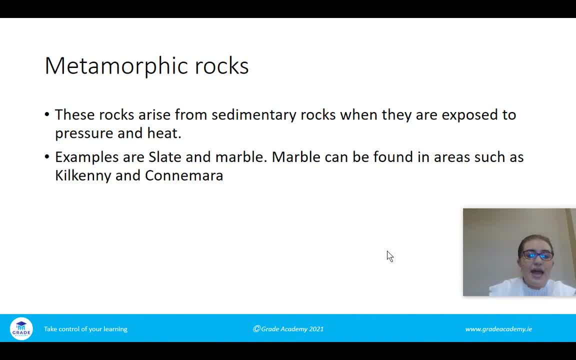 that makes. then you're going to have metamorphic rocks forming and examples are slate and marble. so I always think M for metamorphic rock, M for marble. so marble is probably the main example of it and you can get marble in different areas such as Kilkenny, parts of Galway. you can get it in Kerry. 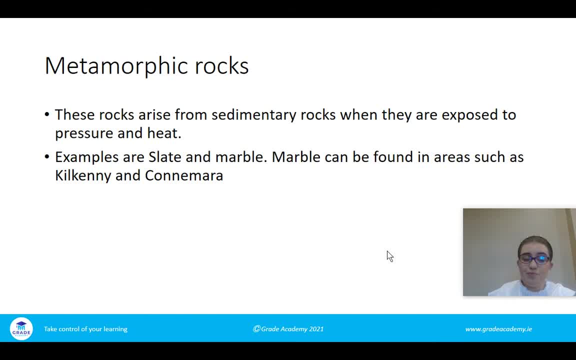 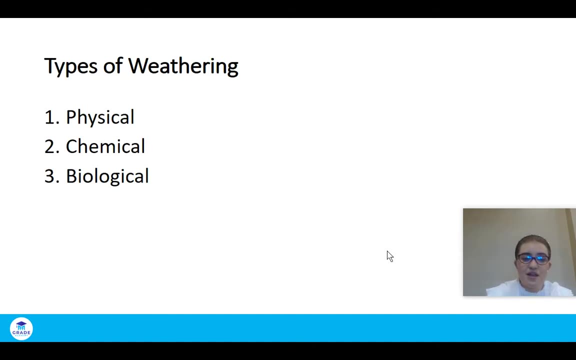 and but it's really really important that you just know very briefly how each rock forms, because each rock- and that forms will have to a degree- will have certain characteristics on the soil that's formed over it. so we have three different types of weathering. we have physical, chemical and 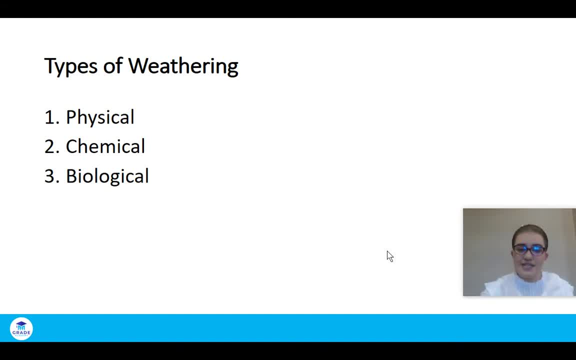 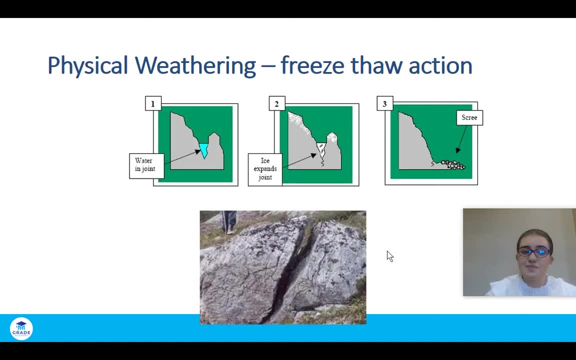 biological weathering, okay. so we're going to look at each of these now for a minute, and we're going to look at physical weathering first of all. the first type of weathering that we're going to look at in terms of physical is freeze-thaw action. okay, so what I've put here is a diagram to explain. 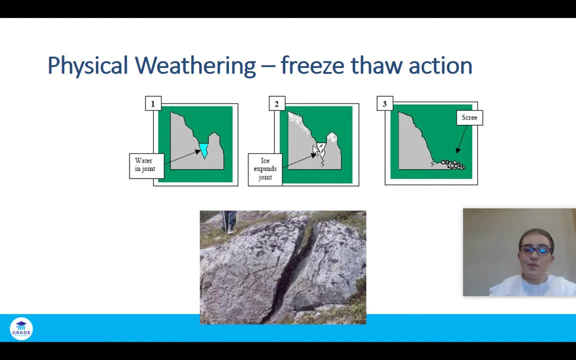 freeze-thaw action, all right, and if any of you do geography, you're probably well familiar with it. but it's fairly straightforward and it is the main type of weathering that we're going to look at, of physical weathering, just for any type of weathering. so the weathering is the breakdown. 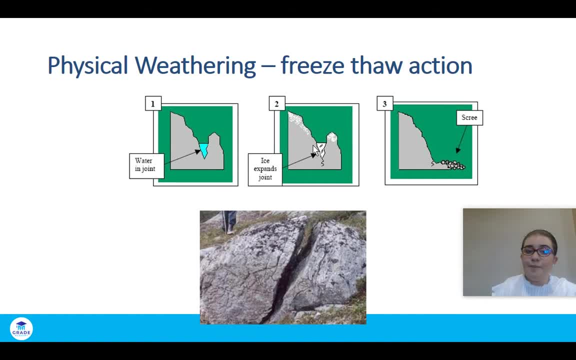 of rock and for any type of weathering. it doesn't happen overnight. it is something that needs to be repeated many, many times. okay, and physical weathering is probably the fastest type of weathering, simply because it's quite harsh. when we look at chemical and biological weathering, they 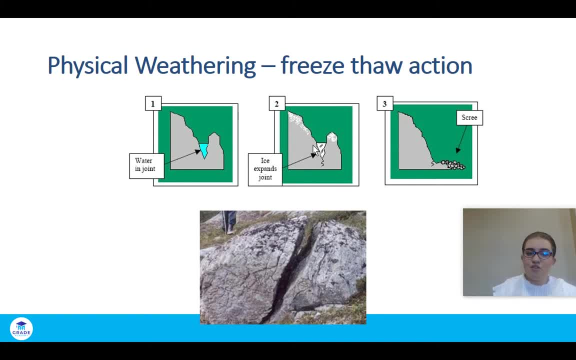 take a lot longer to weather the rock, and why we need to weather the rock is because we need to break down the rock into smaller particles, to introduce that to the soil, and so, therefore, it's going to influence the the soil characteristics. so what happens with freeze-thaw action? so what we? 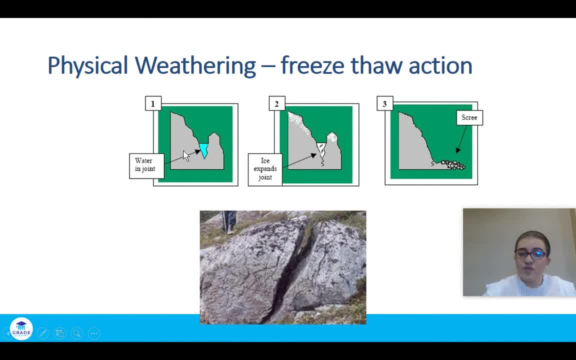 can see in diagram one is that naturally, over time, due to pressure and due to weather conditions, cracks will appear in rocks- so you can see one of them here in the photo- and so water will eventually go into that rock. when we have lots of rain and lots of precipitation, water will go into 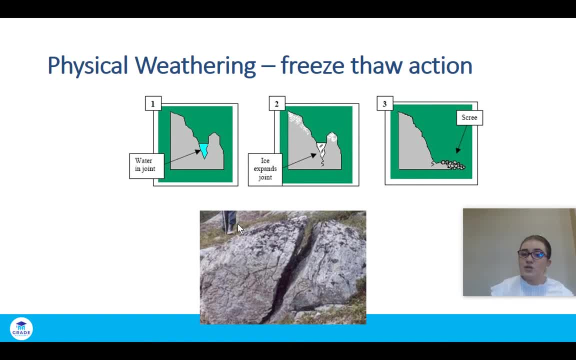 that crack. we need obviously very low temperatures for freezing and we need very low temperatures for freezing and we need very low temperatures for freezing and we need very low temperatures for freeze-thaw action to happen. so really it's only going to happen in cooler times of the year. but 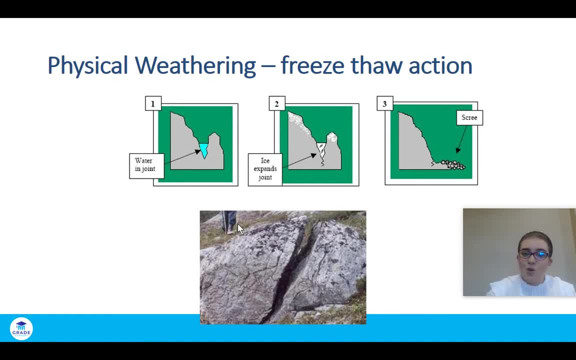 when water enters the rock, ice is going to form, and when water freezes, it does expand. so the ice will expand and what will happen is, because the ice is actually bigger than the area that it's in, little cracks are going to form and we call those hairline fractures, so you can kind of see them. 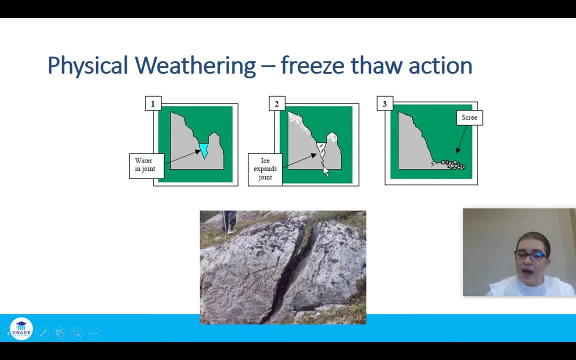 here small little cracks and then by day, what's going to happen is this ice is going to melt the next night. what's going to happen is precipitation is going to um move into that, um kind of crack in the rock. it's going to um freeze and then another crack is going to form. 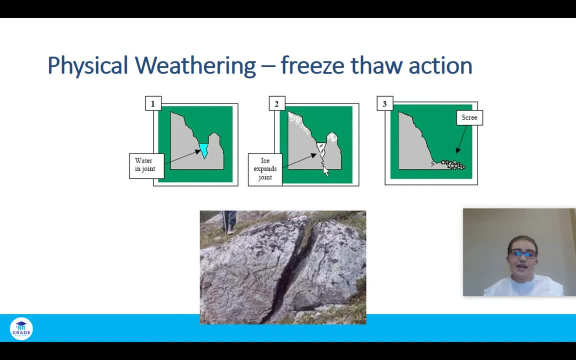 and constantly you have this: ice is freezing, it's melting, it's freezing, it's melting and every time it's doing that, more cracks are appearing in the rock and eventually what will happen is the rock will break away and you can see that over here in picture three. so the rock will actually eventually 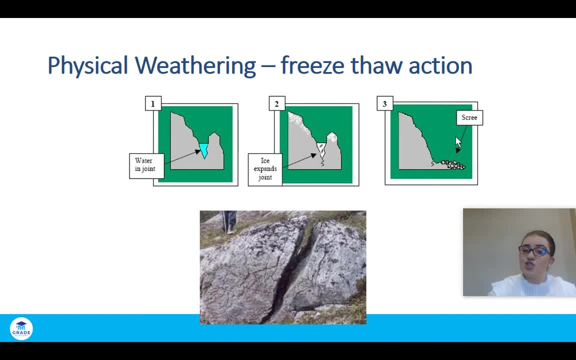 break away into small particles and we call those small particles, the small particles that are in the rock, is called scree. okay, and and over time they will be broken down by weather such as wind, rain, precipitation, and and they will, you know, eventually form um, i suppose, and be embedded in the soil. so 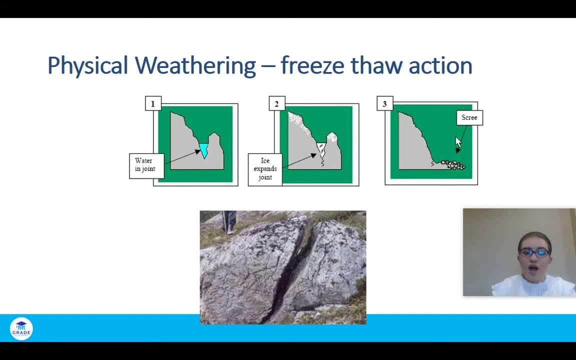 that's freeze saw action. and again, for each of these, i would choose two or three of them, know the names of the physical weathering, be able to write a sentence, a sentence about each of them. that's really, um, what would be required. so other examples of physical weathering. then let's say: 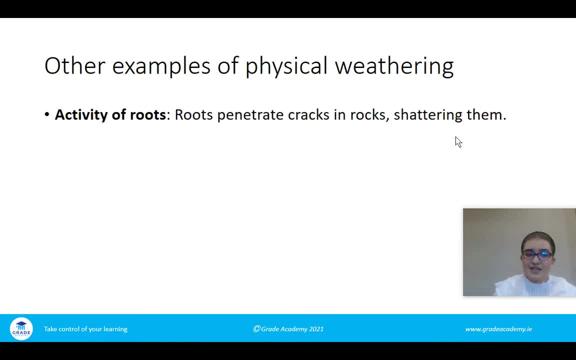 let's have a look at these. so activity of the roots is the next one. all right, so obviously roots are really important in plant growth. depending on the size of the plant, different roots will, um you know, be different strengths and different lengths, so roots can penetrate cracks in. 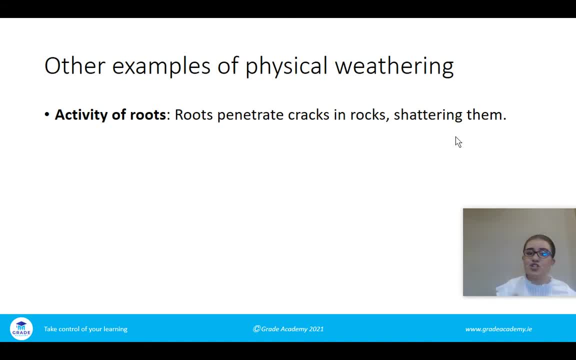 the rocks and they can shatter them. now obviously this is roots of, i suppose, large trees, but again, the larger the plant, the larger the root and so there's more kind of pressure and they can kind of push through a little bit more. and activity of animals. so when we have animals burrowing, 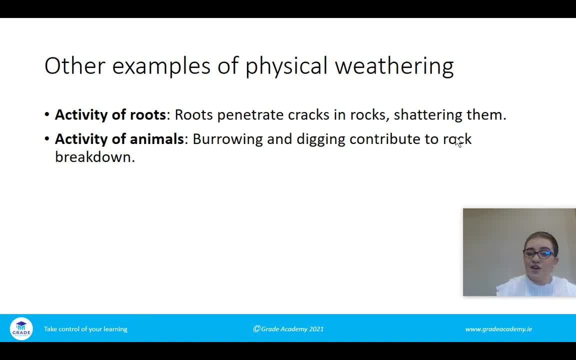 and digging um through stone and through rocks. they are going to eventually break down and even if we have a situation where we have exposed rock and we have animals actually walking on it, that over time is going to break it down again. it is going to be a slow breakdown but nevertheless they. 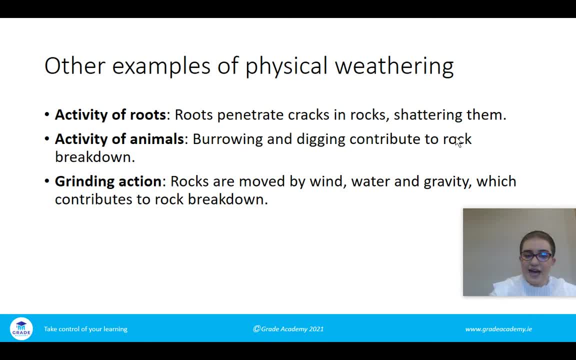 are going to break it down. we have the grinding action of rock. so when we have small particles and we call those scree, when we have those kind of rubbing off each other and rubbing off larger area of the rock and by wind and water and all of those kind of, 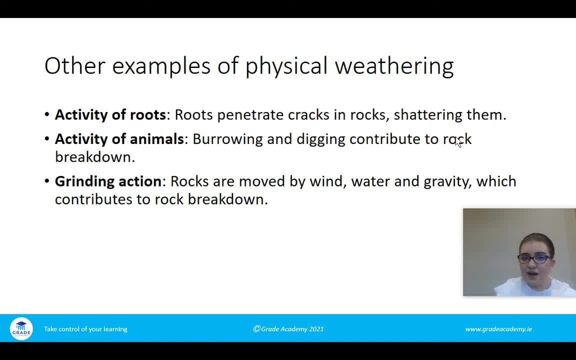 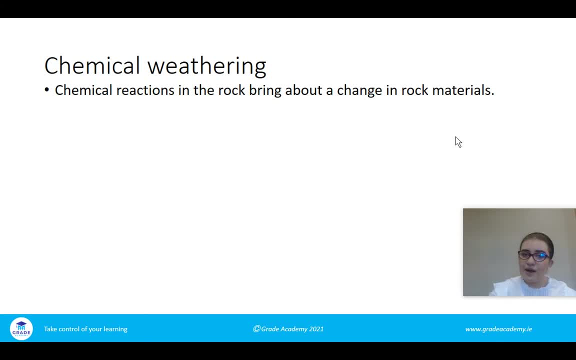 elements associated with the weather that is eventually going to break down the rock and but again, this is a very slow process. so then, looking at chemical weathering. so chemical weathering, um, as i said, is quite a slow um reaction and it's a chemical reaction. so we're. 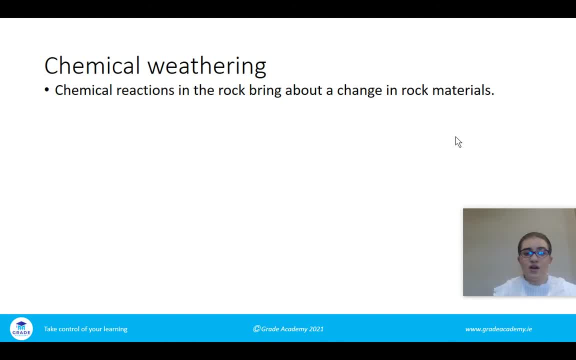 looking really the chemical reactions that occur within the rock to break it down. and why do we need to break down the rock? and i know i keep saying it, but it's really, really important: we need to keep breaking down the rock so that we can break it down and we can break it down. 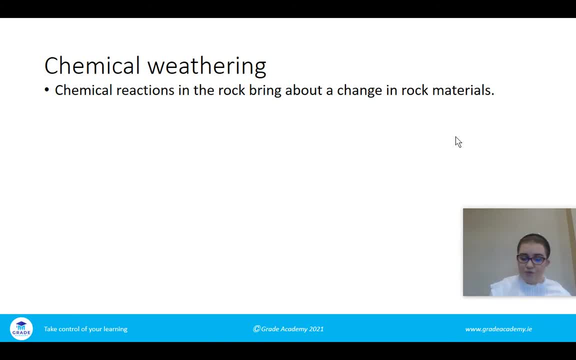 we can embed it into the soil and so that can help with the soil structure. okay, so looking at a few examples here for chemical weathering. so the first thing is we have hydrolysis- okay, so hydrogen ions in the water. so water is made up of h2o, so hydrogen and oxygen in the water will react with. 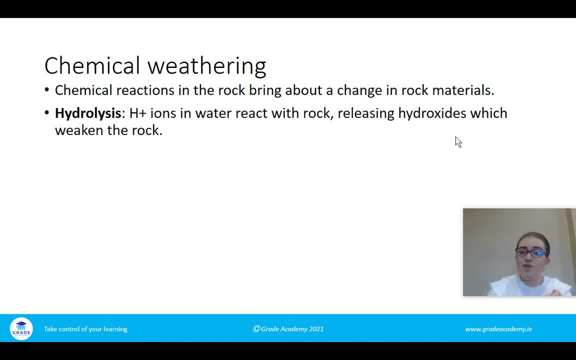 the rock. so where does water come from? well, it comes from precipitation it comes from, which is anything that falls from the sky, so like rain and snow, and so there is going to be a huge abundance of water. so when the hydrogen ions in the water react with the rock, they will release hydroxylites. all right, 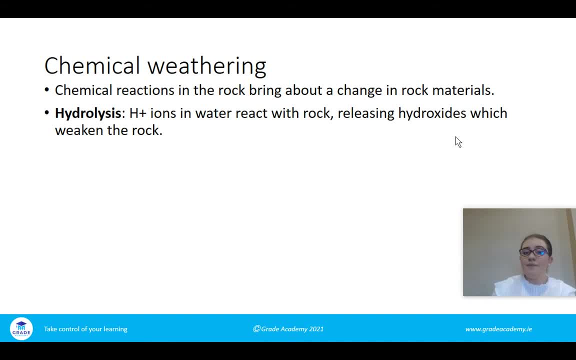 what they are. they are chemical and they will. just over time, they will weaken the rock and when they weaken the rock, eventually they are going to break it down. hydration is the next thing. so, if you think about it, why do we drink water? to be hydrated. so it's the same principle. it means the same thing in. 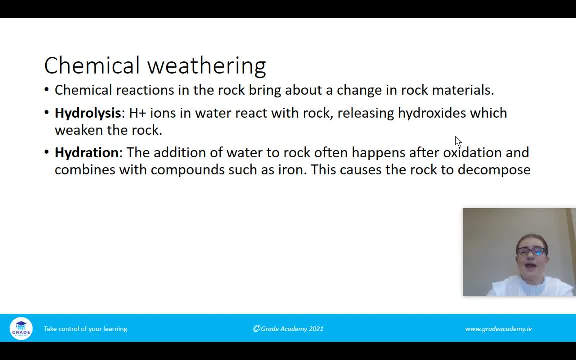 rock. so when we add water, we are going to have, um, you know, certain elements in in um rock and one of those is iron. so iron is a really common element in rock and therefore in in soil. and so when we add water to rock, um, and when there's iron present, 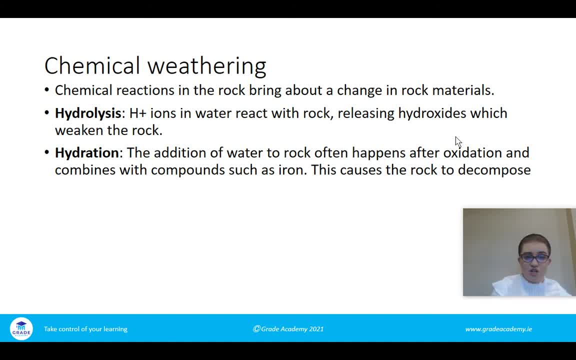 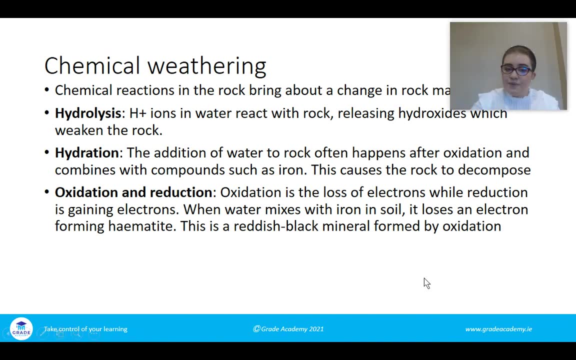 in it. this will the mixture, I suppose really, of the water and the iron in the rock will cause the rock to break down and to decompose. okay, the next thing, then, is oxidation and reduction. the way I always think of this is oil rig. so oxidation is the loss of electrons. reduction: 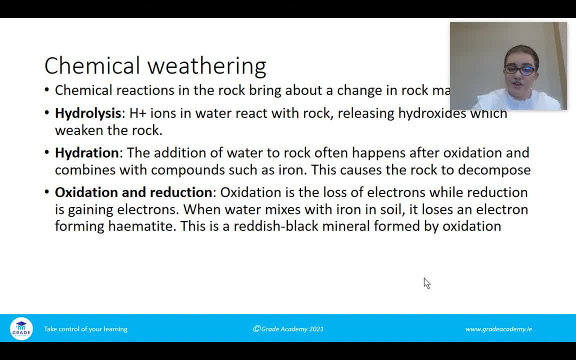 is the gain of electrons. so if any of you do chemistry you'll probably have heard of that already. but oil rig is for oxidation reduction. so oxidation is the loss of electrons. so all um living and non-living things have um particles in them and there there is always the movement of 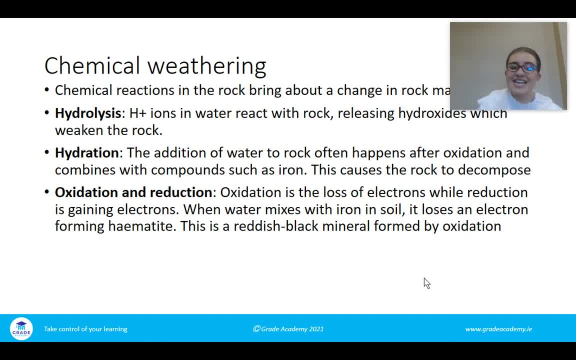 electrons in the movement of particles. so oxidation is the last of them. reduction is the gain of water mixed with iron in the soil. it will form a hematite. So that's really, really important to know that term. That is a reddish, black material And that again will form kind of 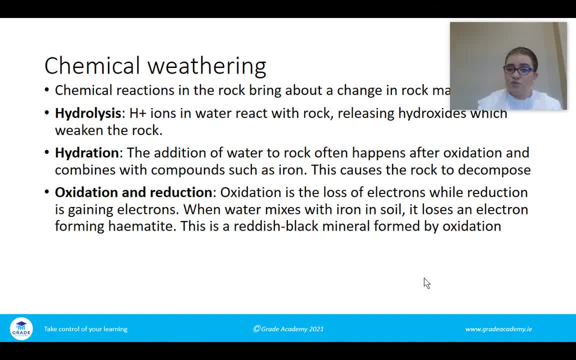 over time and the more hematite that forms, it will cause the rock to break down. Okay then the final one is solution and carbonation. So when water dissolves, or water dissolves minerals as it flows through the rock, if water combines with CO2, which is very common in the 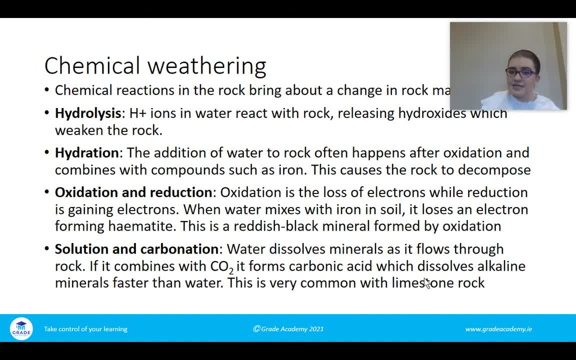 atmosphere. so therefore it's going to get into rock. it will form carbonic acid And carbonic acid. so how is that formed? That's when water will mix with carbon dioxide, So that will form carbonic acid and that will break down certain types of rock. That is very common with the 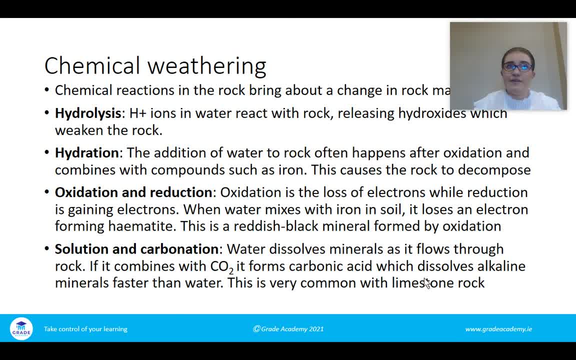 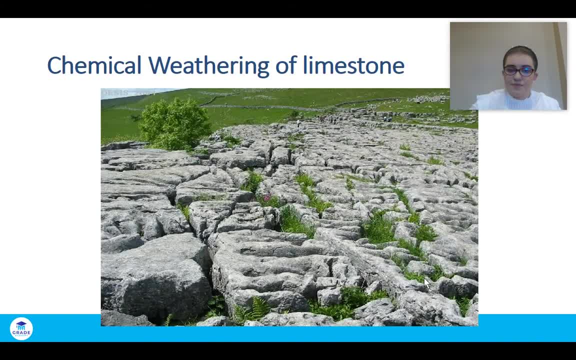 limestone rock. So when we have exposed limestone, like in areas of the burn or any area really where you have limestone, you are going to break it down, Okay, So you can see it there, So you can see lots of. so that's an area of the burn and you can see lots of weathering there, lots of. 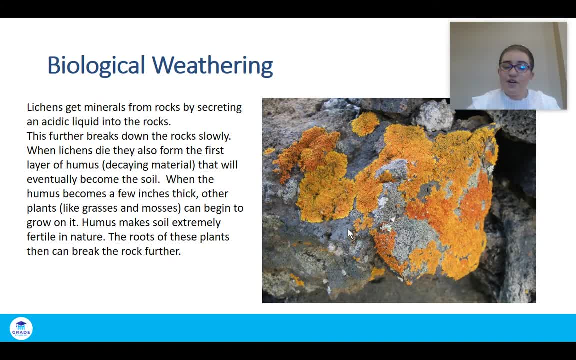 breakdown of the rock. So biological weathering, then, is the third type of weathering, And what we can see here in the diagram is we can see lichens. Okay, So lichens are part microorganism, part plant, And what they will do is they will attach themselves to rock. 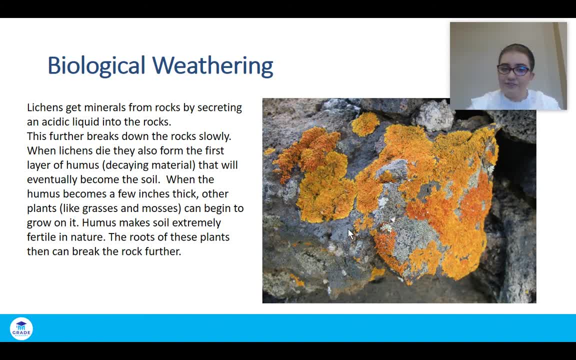 So a lot of the time when we see this on rock, we think it's not living. It is living And what they will do is they will break down the rock by secreting minerals into the rock, And the reason that they'll do that is because, well, it's breaking down the rock first of all, but also 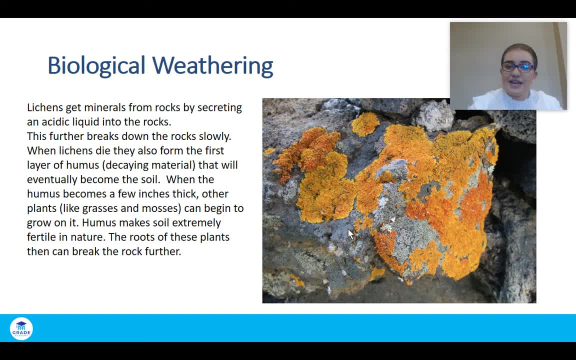 in the rock there is going to be certain minerals And when the lichen can secrete in those chemicals they're going to get back some of the minerals. So it's really kind of helpful for that. So they get their minerals by secreting in an acidic liquid into the rock. 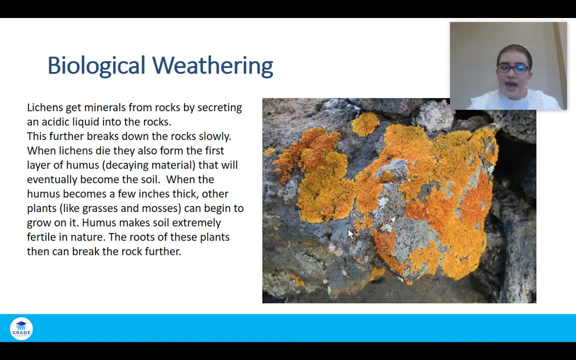 And this will break down the rock, but it's a very, very slow process And it does take quite a long time for the lichens to actually break it down. Lichens are also really important in so that's how they're going to break down the rock. but they're also really important because 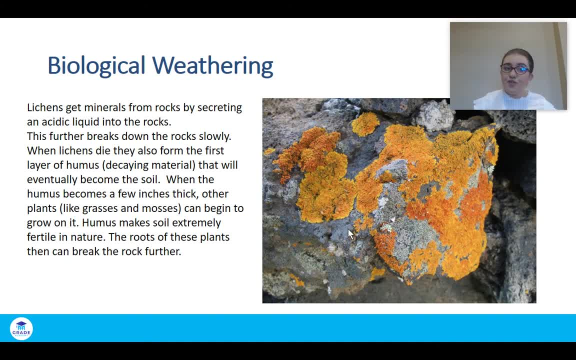 they are a living organism. So when they die there is still going to be a certain amount of minerals and nutrients in them. So what would happen is that would actually. so when they die they kind of dry up and they actually fall off the rock. When they fall off the rock, they kind of 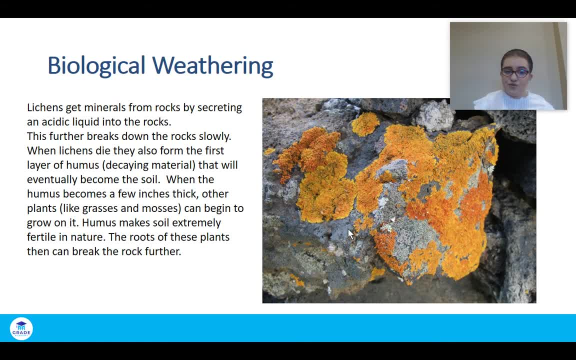 go into the soil And when they mix in with the soil, they're eventually going to form humus. Humus is, you know, the remains of dead animals and plants that have been compressed over time, And that's really, really good for in terms of the fertility and the nutrients of the soil. So 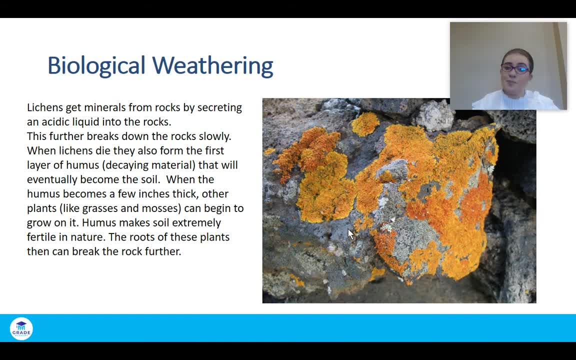 I have it there. It's really, really good. And how you would know that a soil has a lot of humus in it is because it's dark in color. The darker the soil, the more humus that's present in it. And 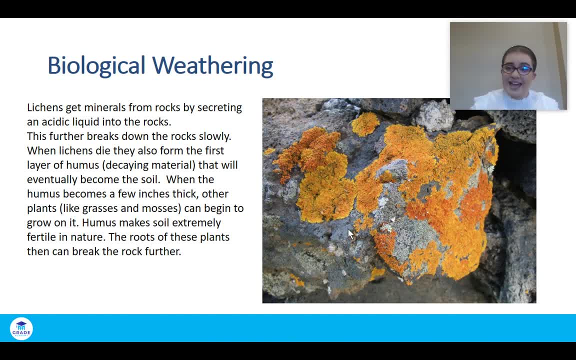 the better it is going to be in terms of fertility. So there are the three types of weathering. Again, name them, write a sentence about each of them. Obviously, for freeze-thaw action and for chemical weathering, you would need to know maybe two examples of each of those. 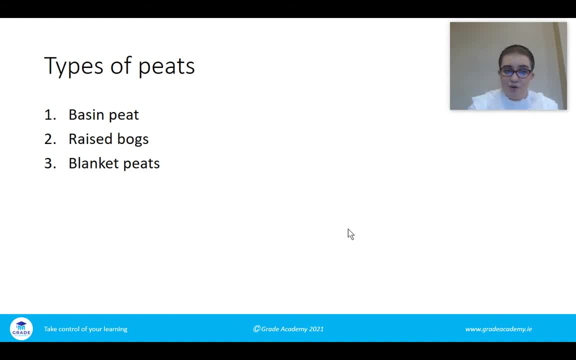 So the next thing that we're going to look at is the type of peat that form Okay. so peat is another word for a bog. So we have three different types of peat. We have a basin peat, a raised peat. 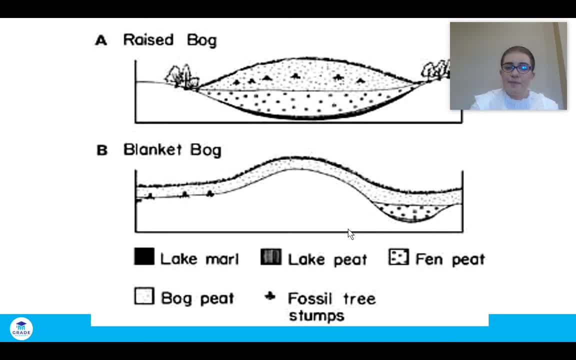 and blanket peat. Okay, so if we look at this diagram here, what we can see is we can see a raised peat or a raised bog. So we can see it here. it forms and if you follow my mouse around you can see it forms kind of like a hill, But initially, before that forms what we 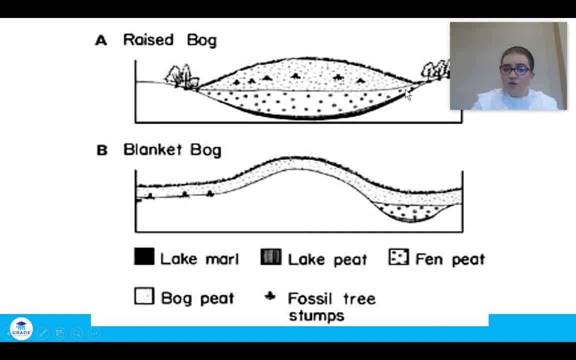 have is we have this depression or we have this hollow here. Okay, so you can see that hollow there And how a bog will form is where you have vegetation and where you have dead animals and plants in this area and where there's generally anaerobic respiration. So there's very, very little. 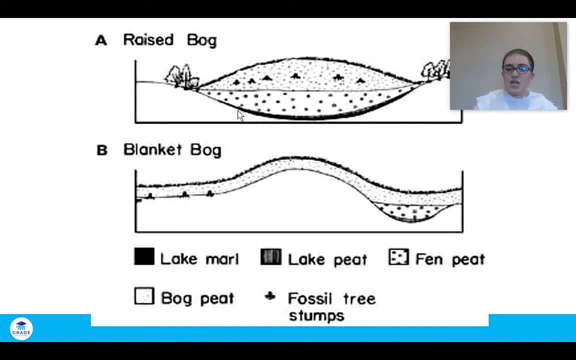 vegetation in a certain area that will kind of break down to form a peat. So the first one that we have is a basin bog. So a basin bog is where we have any kind of depression, so like a valley lake, anything like that, a lake that has dried up and you have vegetation added, adding to it. 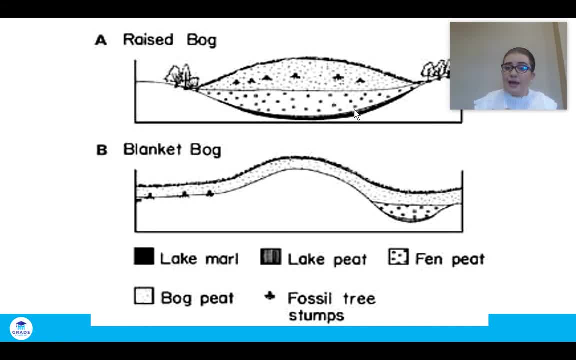 Over time. when you are adding vegetation to that, it's going to form a basin bog. Okay, when we continue to add vegetation and this will just happen, like very, very gradually over hundreds and thousands of years and due to weather conditions and animals and things like that. 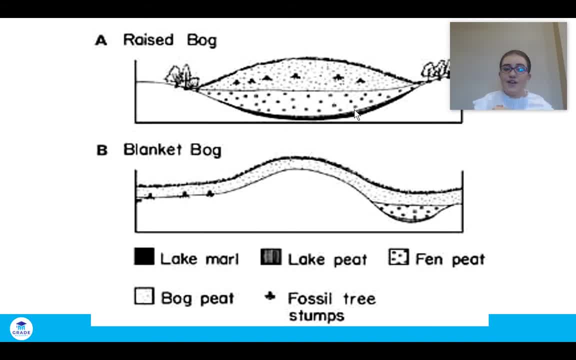 animals and so on and so forth. But when we have vegetation being added on top of a basin bog- what we call that is a raised bog- Okay, so you can see it here- it's kind of like a hill. Then when we have vegetation on either side of that basin bog, it kind of nearly levels it out. 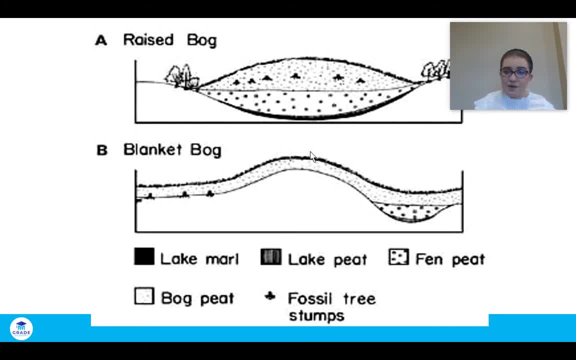 and it levels it out to quite a thick area and we call that then a blanket bog. So what's important for each of them is just to know how they form. So again, basin bog forms in the section just by the adding of vegetation. A raised bog is just an extension of that. 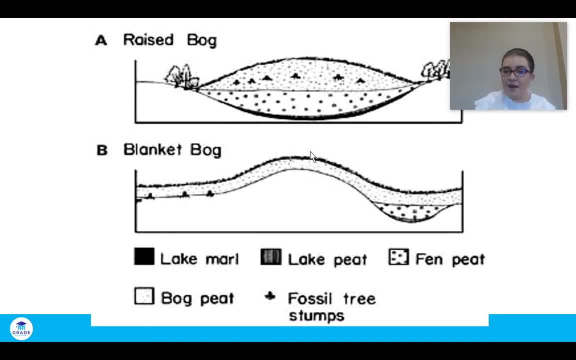 and then a blanket bog is where you just have built up a vegetation on either side really of that kind of hill And a lot of the time for bogs or for peat there would be very, very little oxygen there, And that is why they are unique to certain animals and plants that 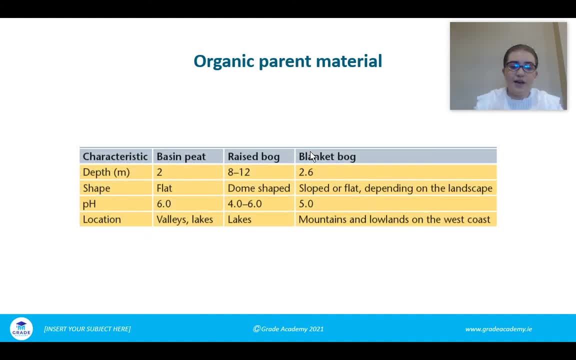 will be there. So, looking at this table, here I have the three types of peat And basically what's important to know is just the depths of them. So I've gone through the kind of shape of them, the depths of them, where they're located, and the pH is quite important. 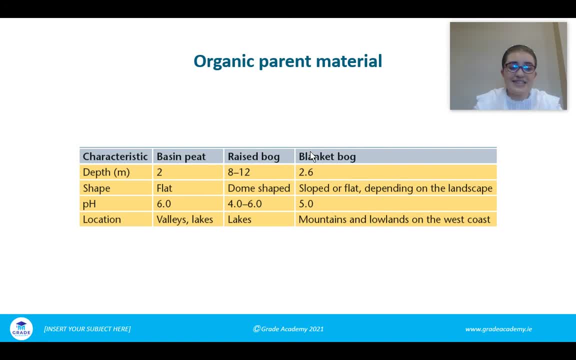 So we'll have a little look at them. So the basin peat first of all, so the depth can be about two meters, So you don't have to be. it doesn't have to be mad deep altogether for a bog, but it's very. 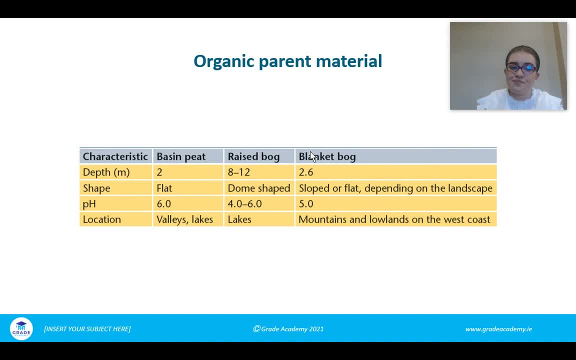 very compressed over time, So there's a huge amount of living organisms that were once living there. It starts off quite hollow but again eventually it is going to turn quite flat when it kind of levels out with the soil surface. The pH is about six And again where you'd find it is in any 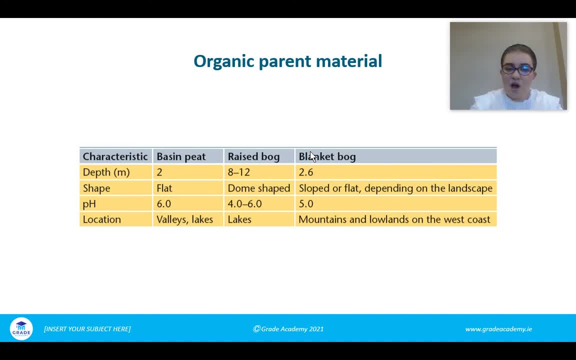 kind of depressions, like a valley lake, something like that. Your raised bog then will be a good bit higher, And so the raised bog is the one that's kind of like a hill. It is that dome shape, and the pH can be a little bit lower, depending on weather conditions, because it's a little bit more exposed. 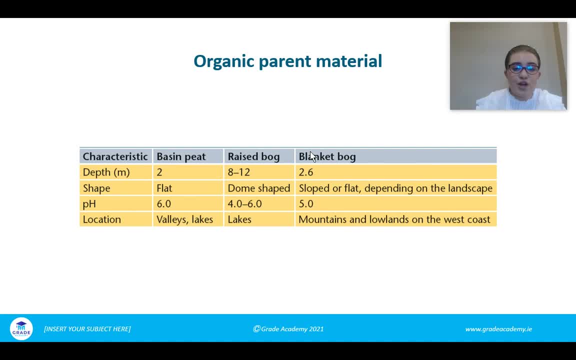 to them. So it can be about four to six. And again, where you would form that, it's formed really really low, it's formed really from the formation of valleys, lakes, but it's just kind of an extension of them, and then your blanket bog can be about, you know, two to three meters. uh, in depth it is quite um. 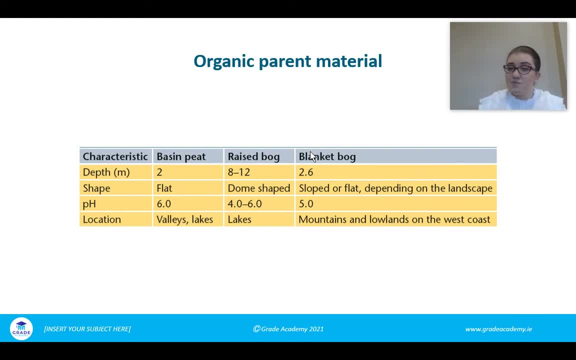 flat and generally where you'd have it is at the kind of the bottom of hills and mountains and just kind of where it levels out, okay, and that's just the the names of them there. so, finally, the last thing that i'm going to have a look at are the factors that 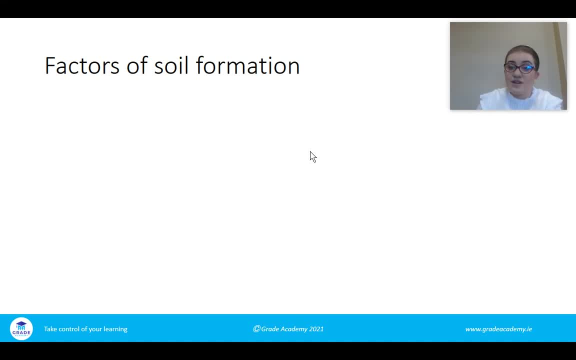 um are important in soil formation and these are asked quite a lot. so there's five of them. i would learn the five of them. so the parent material is the first one. so the parent material is the type of rock really that it comes from and that makes up 45 percent of the soil and and it will influence 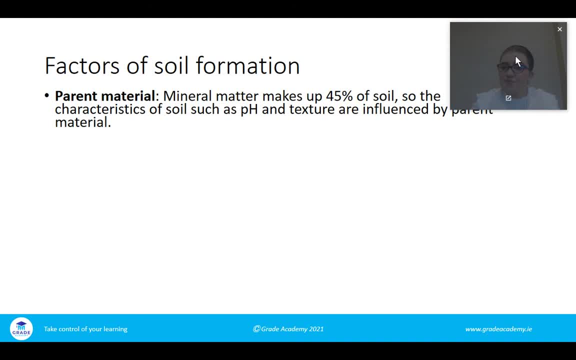 certain characteristics, such as the ph, the texture of the soil, lots of different things like that. so um, the ph, um of the soil texture, directly influenced, really, by the rock that, the parent rock that's underneath. okay, the next thing, then, is climate. so temperature and precipitation will contribute to the wet. 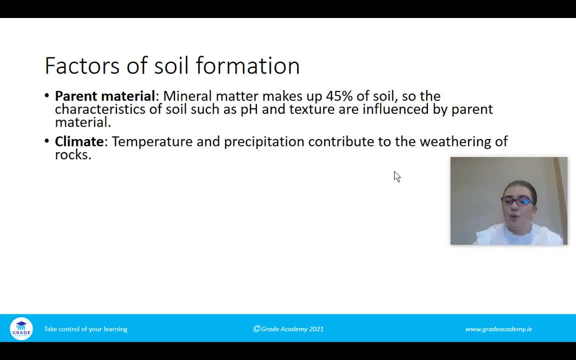 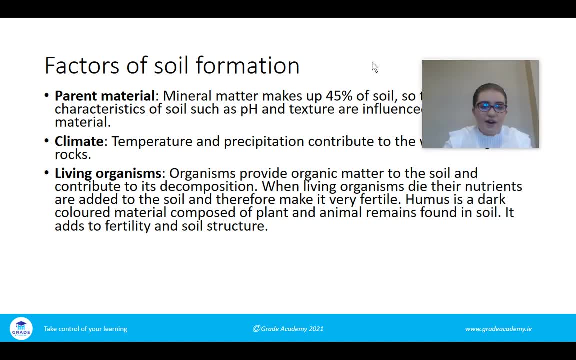 weather in your rocks, especially precipitation. so we've got a freeze action, we've got wind, rain, and all of that is going to have an influence on rock. living organisms are going to influence the rock and because when you have living organisms, so they might be microorganisms, they're going to 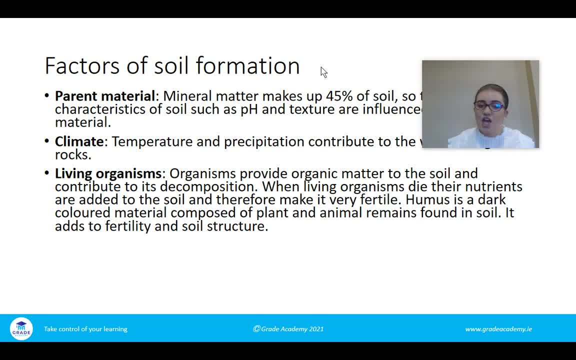 help to break down the rocks, so the bacteria and fungi have decay. you also have earthworms there. earthworms: what they're going to do is they're going to move through the soil, um, and they're going to form little channels to allow air through, but also when you have any. 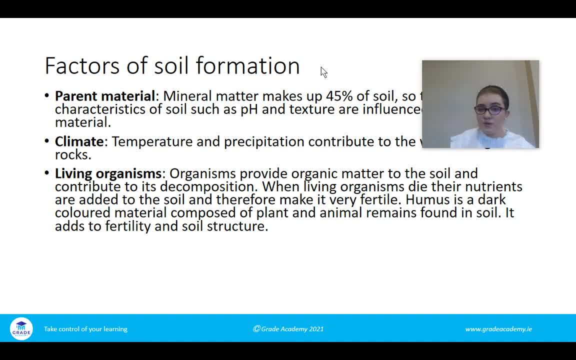 living organisms, whether it's animals or plants, when they were once living, and when they die, they are going to break down in the soil, and when they break down in the soil, they are going to form humus, and humus is something that will add to fertility and soil structure. 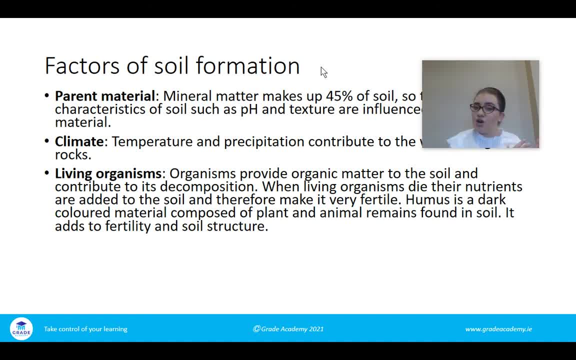 and why it adds to fertility is because there's the nutrients from your once um living organisms. they have obviously now broke down, but there's still those nutrients there, so the soil is going to get some of that, and humus also adds to soil structure because it creates this crumb structure. 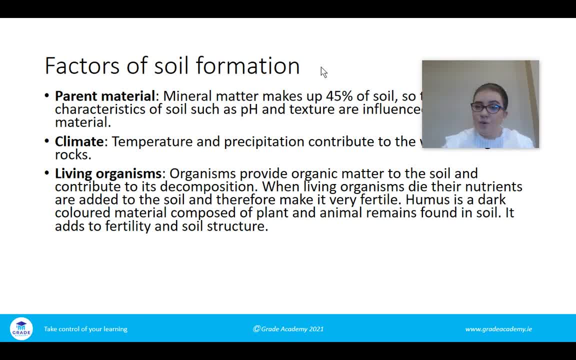 so if you look at any soil type and you can break it up into like little bread crumbs, we would say that that soil is very, very fertile. okay, topography then is the slope of the land. so where you have very, very steep slopes, like mountainous areas, you are going to have a lot. 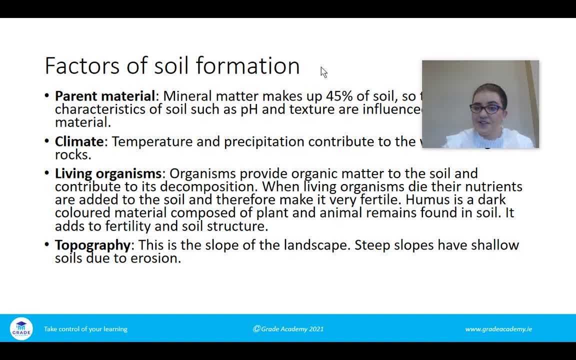 of erosion, because you're going to have high um wind activity and high rain. there, you know, the conditions are much harsher and the higher the altitude. and then, finally, the last one, is time. so irish soils are quite young, as they were formed after the ice age, and so that has. 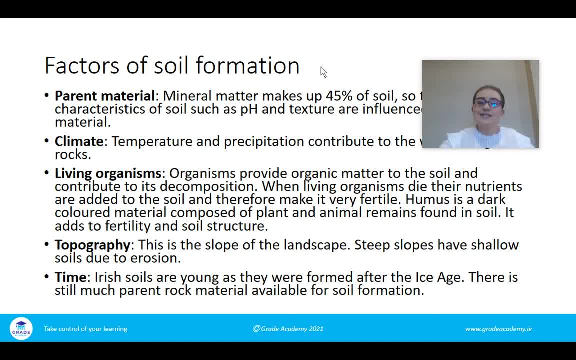 obviously a lot got to do with the soil formation. so that is the first little part about soil formation. in the next video, what we'll have a look at is the classification of soil, so the different soil types, and what we'll be doing is we'll be looking at the diagram or the soil profile. 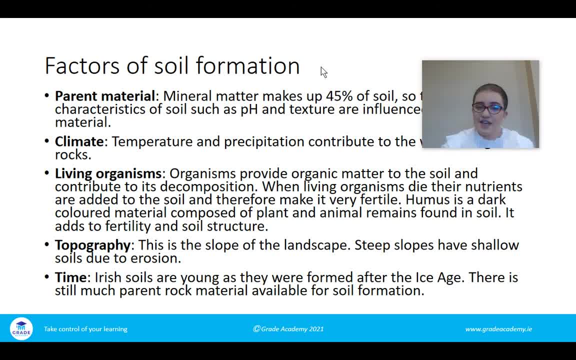 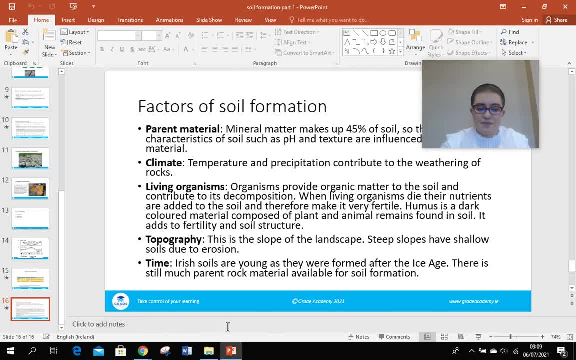 for each of them, okay. so thank you for listening and i'll see you in the next video. bye, bye and until the next time. happy learning.